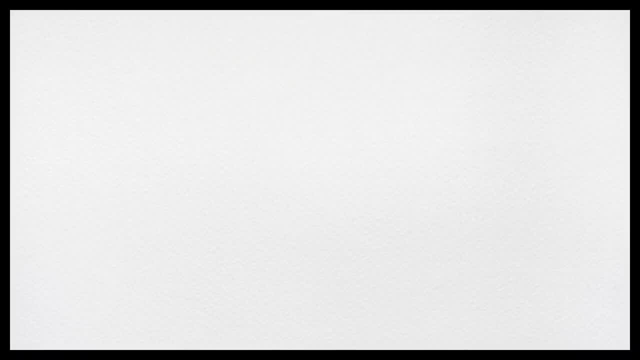 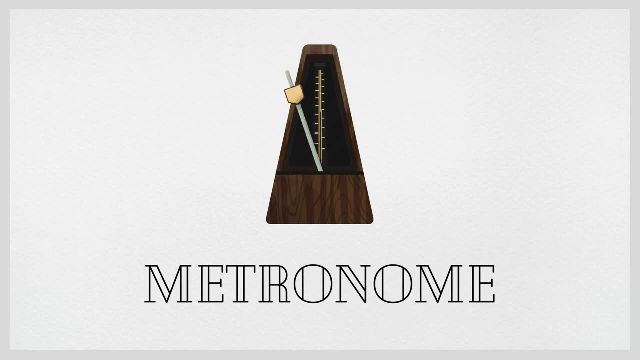 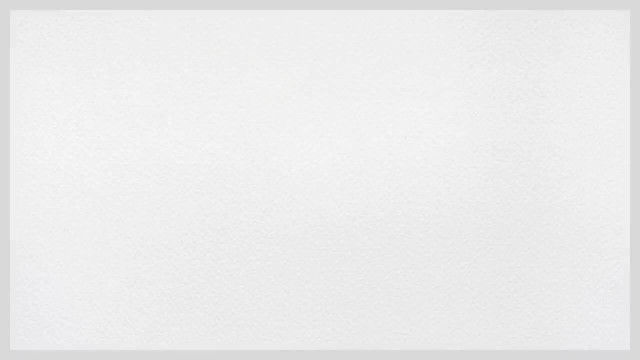 What you are seeing and hearing right now is a metronome. The job of a metronome is to set the tempo for music. Because of this, the metronome is the basis of all music. The current tempo you're hearing right now is 120 beats per minute, or BPM. This means that the 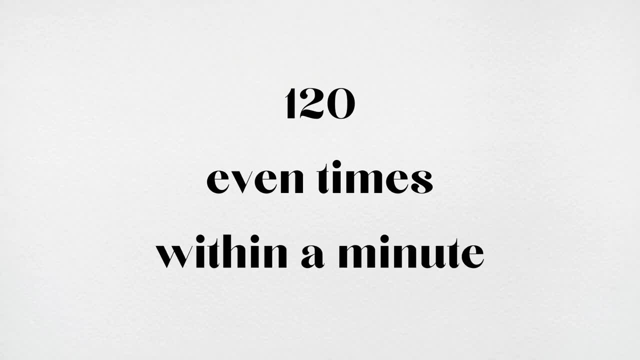 metronome will click 120 even times within a minute. Now, not all music is played at 120 BPM. Music can be played at any tempo. We'll talk about that some more in another video. For now we'll stay at the common tempo of 120 BPM. 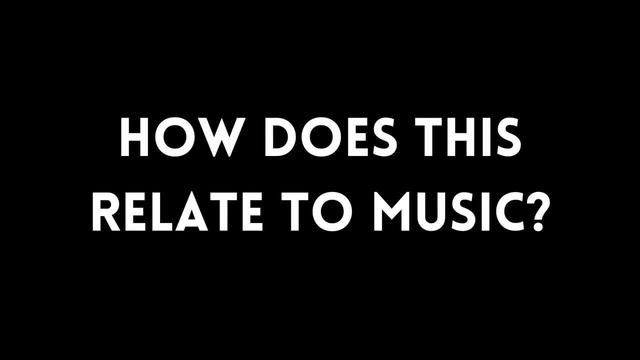 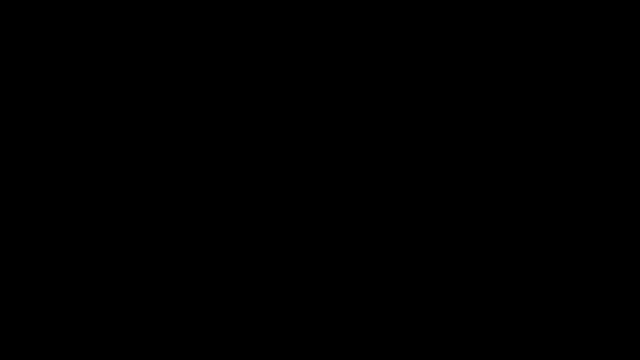 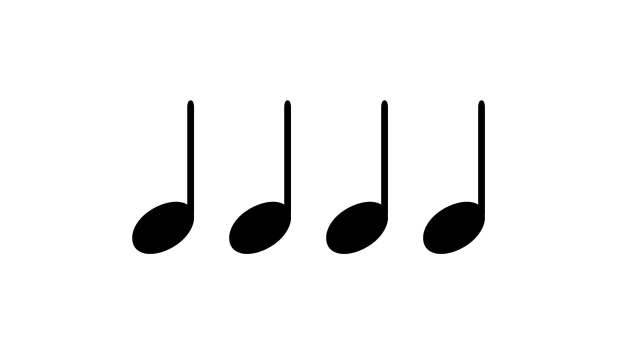 Now you might be wondering how this actually relates to music. I'm sure almost everyone has heard of music having a beat or a tempo, but what does that actually mean? This is a quarter note. Usually, when we talk about tempo, each one of the beats you heard earlier would represent one quarter note. 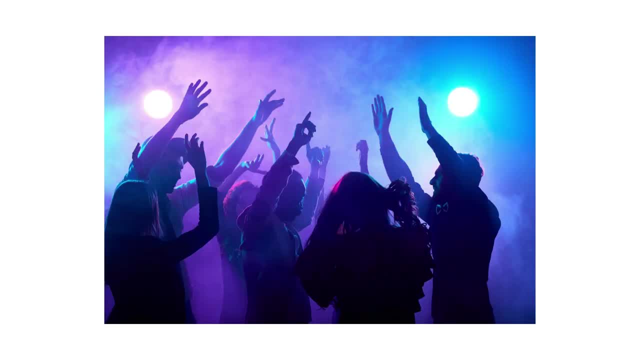 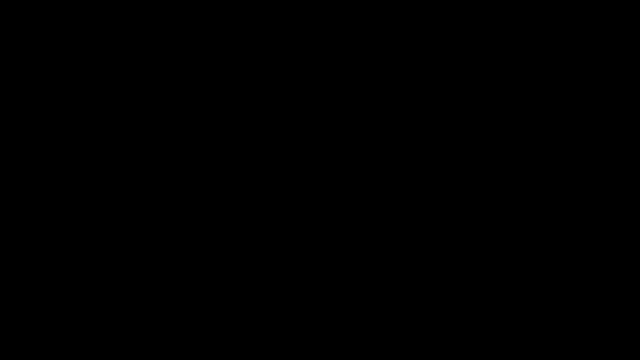 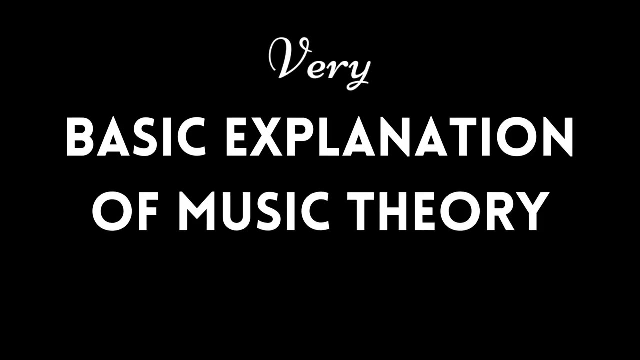 This is most oftenly what people feel or move to as the beat of a song. Before we move on to explain different types of beats and note values, it is important that I state that this video is a very basic explanation of music theory. There are several variations in music over time. to Knowing century for Japanese music. 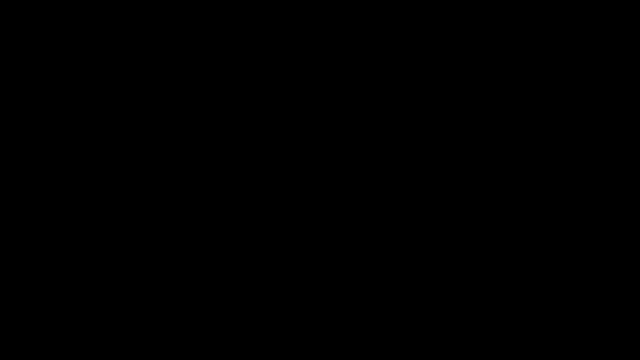 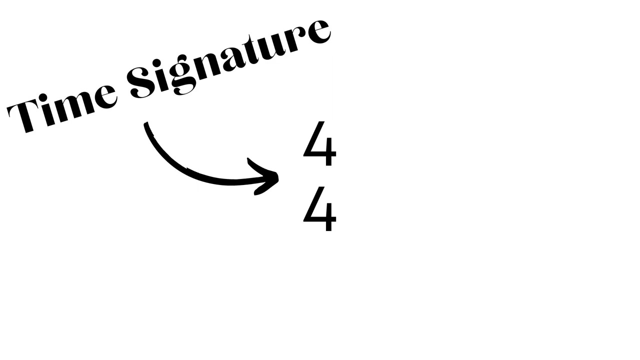 and there are some differences due to the type of music that was created, So these does not really help us. while making this Video easy. once we are on to the rest of the way, This is called a time signature. The number at the top of this bill shows sempre MARK. 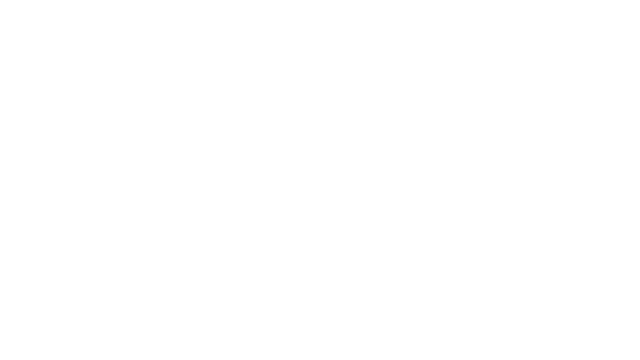 how many beats are heard by a measure, while the number on the bottom of the bill shows what note is heard. A measure usually works on a single note, but usually only on the answer. It's usually called a beat sound, used to help musicians keep track of rhythm by dividing sheet music into organized sections. 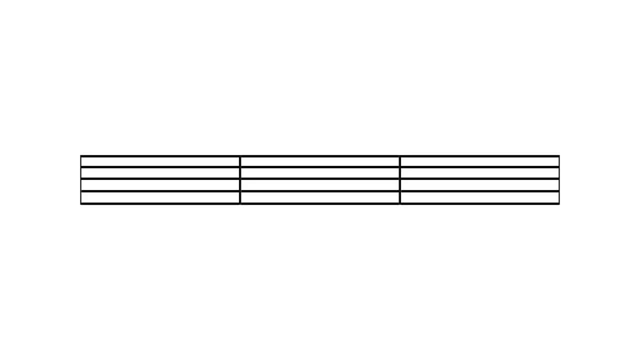 They also give a sense of pulse to the music. Measures are indicated by a vertical bar separating them, and the length of a measure is determined by the time signature. Before we continue further, it is important to explain the different notes, values and beats in music. 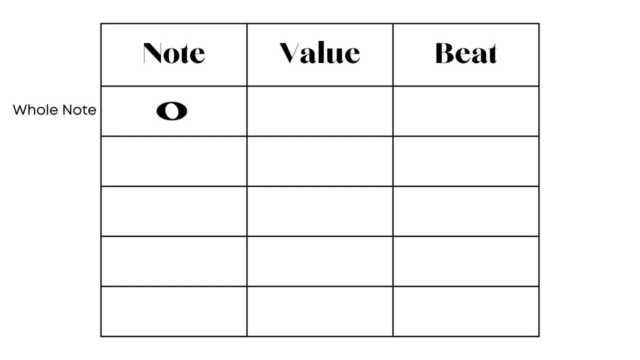 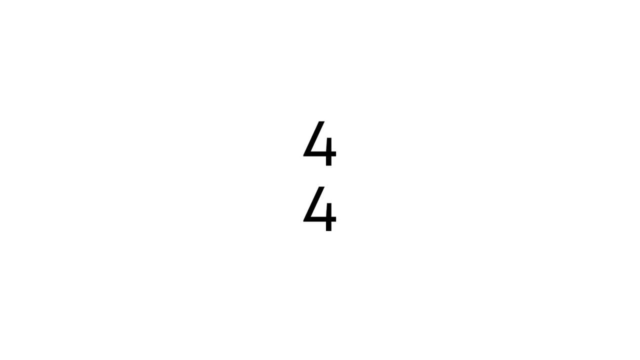 The five most common types of notes seen in music are the whole note, the half note, quarter note, eighth note and the sixteenth note. For now we'll use 4-4 time to explain, as 4-4 is the most. 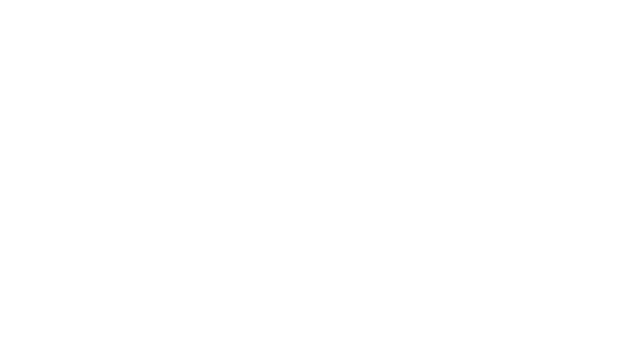 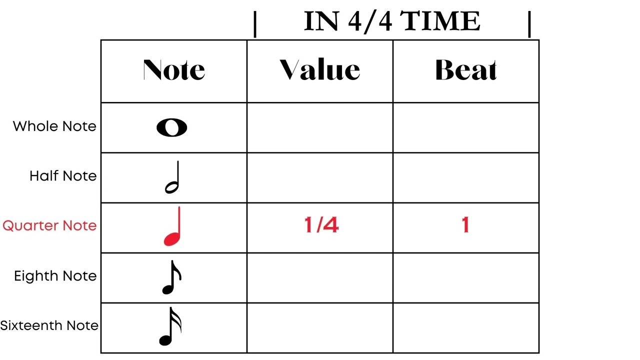 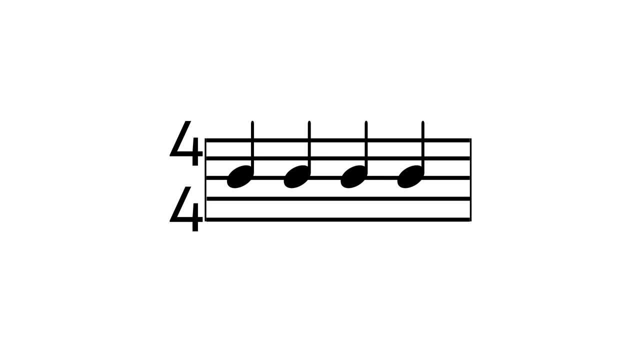 common time signature seen in music. In 4-4 time the quarter note gets the beat. This is because the quarter note has a value of 1 over 4.. The bottom number of both the time signature and the value of the note are the same. so four quarter notes will fill up one measure in 4-4 time. 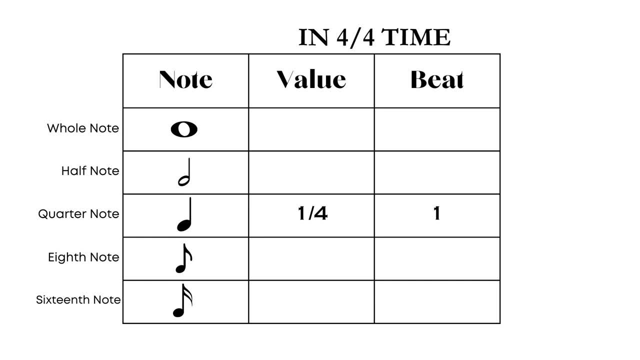 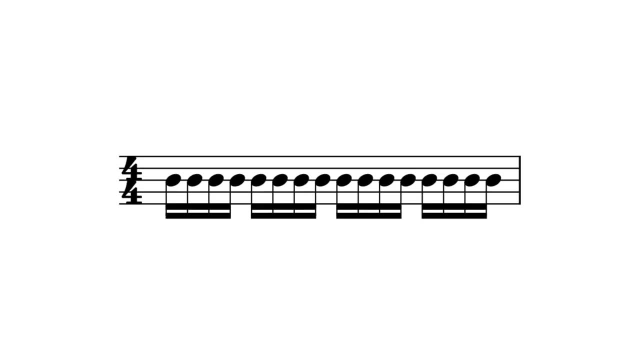 Based off of the chart from before, we can now determine: 1- Eight eighth notes are required to fill a measure of 4-4 with eighth notes. 2- Sixteenth, sixteenth notes are required to fill a 4-4 measure with sixteenth notes. 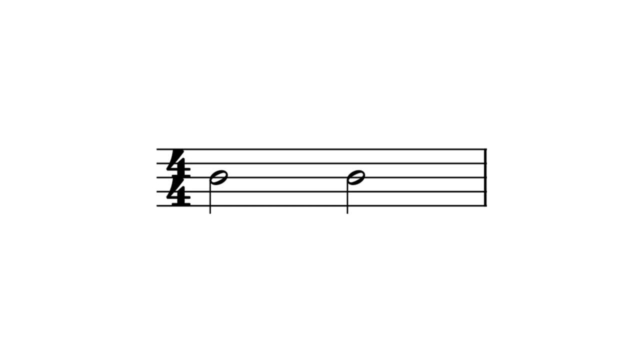 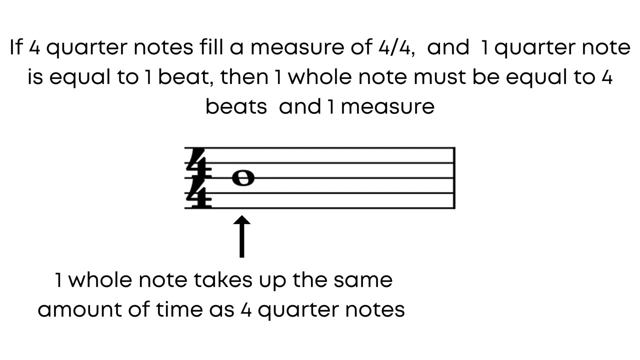 3. Two half notes are required to fill a 4-4 measure with half notes. 4- One whole note is required to fill a measure of 4-4 with whole notes. Now, if you didn't get the answer to the question, 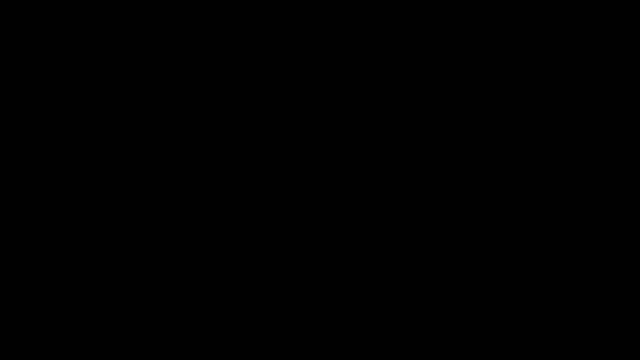 I don't blame you. I used a very mathematical explanation of the relationship between those five types of notes. I feel that explaining notes this way makes it much easier to understand the relationship between note values as we get more complicated. If you didn't understand, 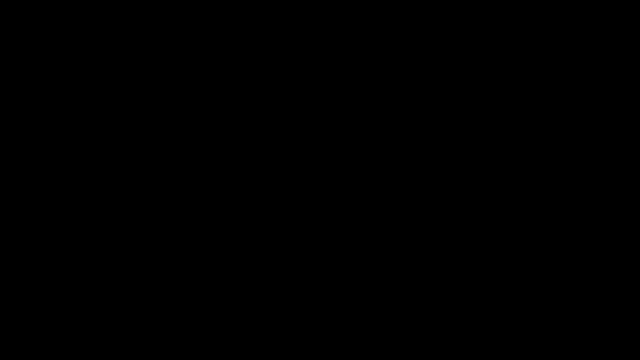 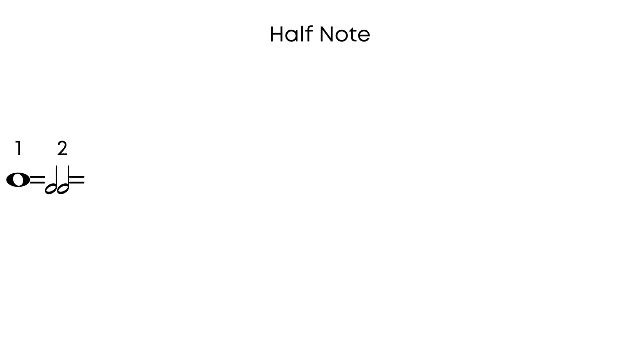 that previous section. it's perfectly fine. The main point of what I was saying about note value relationships is the following: One whole note takes up as much time as two half notes, which take up as much time as four. quarter notes, which take up as much time as eight eighth notes. 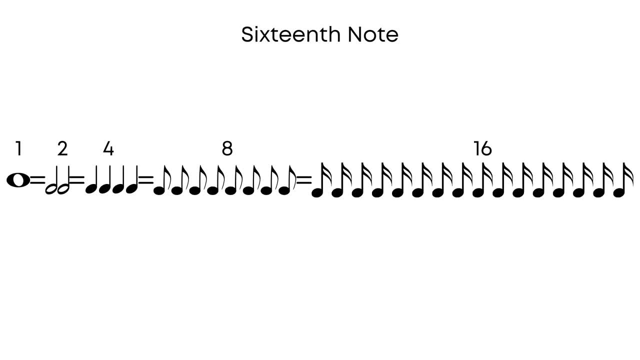 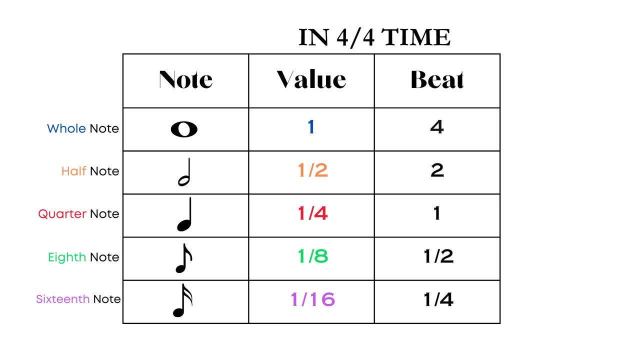 which take up as much time as sixteen. sixteenth notes. If you haven't already noticed, there is a relationship between the names of the notes and how they fill up a measure of 4-4. With 4-4 being the most common time signature. knowing the. 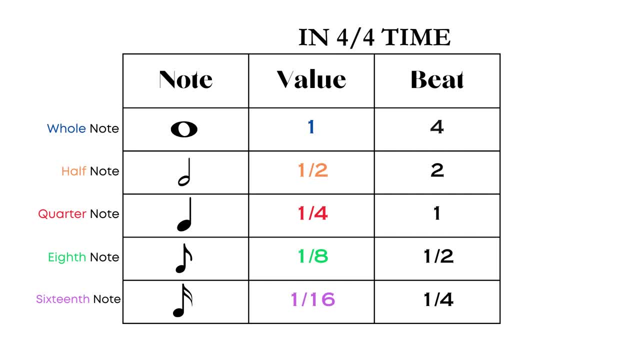 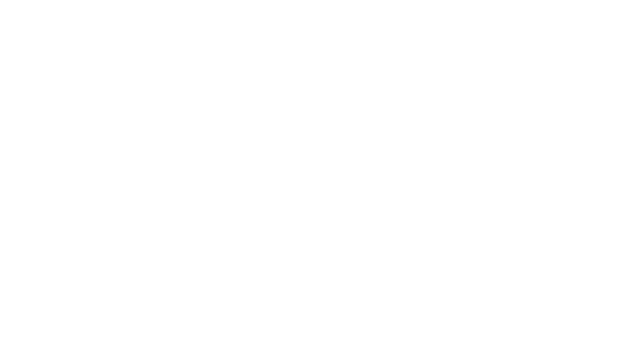 names of the different notes will be very helpful in remembering how notes function within sheet music. The final topic we will discuss in this first video is an introduction of clefs. We will go more in-depth with the introduction of clefs later in this video, but before we do that, let's 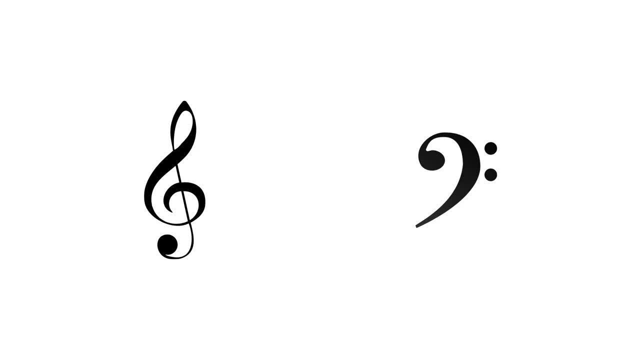 take a look at some of the clefs we will be discussing in depth with reading pitch in the next video. Clefs show musicians the position of notes on the staff and they are required for musicians to be able to read sheet music. The most common clefs seen in music are the treble clef.